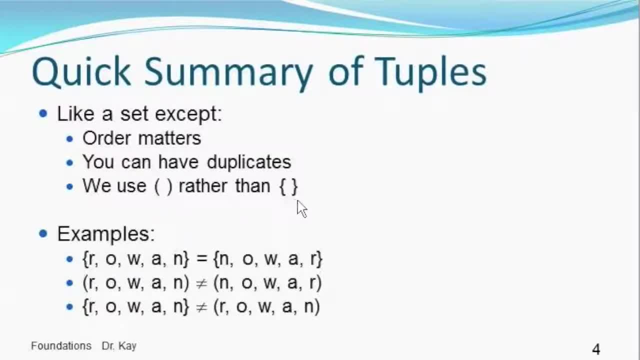 of them, and we're going to use these regular parentheses rather than curly braces. So, for example, we might have the fact- here's an old fact that you should know- the set R-O-W-A-N is exactly the same as the set containing the elements N-O-W-A-R. That's fine. 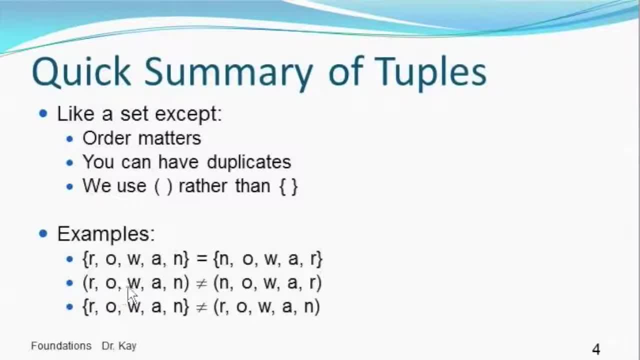 but if you have a tuple with R-O-W-A-N in it, that is not the same as the tuple with N-O-W-A-R in it. Of course we know this is a tuple because of the parentheses there. order matters and and the elements in this tuple do not appear in the same order And sets and. 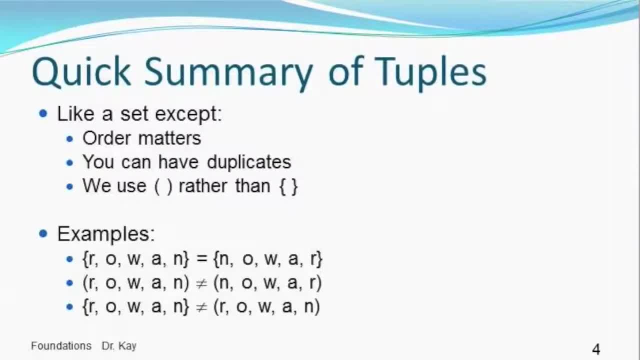 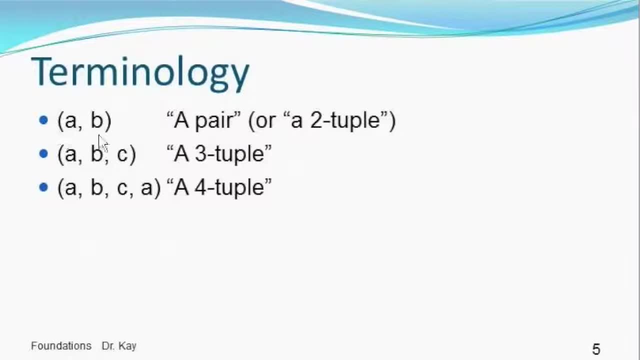 tuples are different beasts. You never have a set equal to a tuple- Some terminology we will often call a tuple with just two elements a pair. Otherwise we might call it a two tuple. Similarly a, a tuple with three elements. We might occasionally call it a triple, but usually it's a. 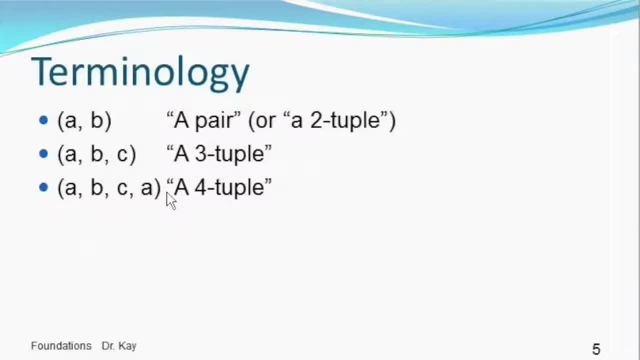 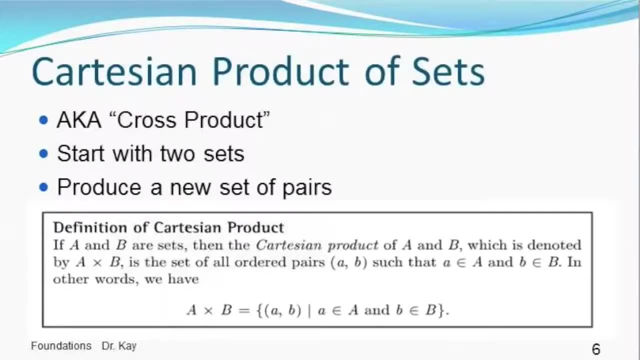 three tuple, And then we just keep going. This is a four tuple, and you can have a 27 tuple and a 56 tuple if you want. Another thing that you should also be familiar with is the Cartesian product of two sets, or the cross product of two sets. You start with two sets and you produce a new set of. 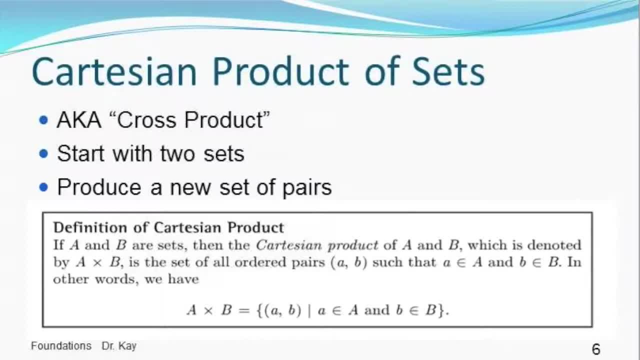 pairs, So a new set that contains elements, each element of which is a, two tuple. So if we look at the definition here from the book, if a and b are both sets, then the Cartesian product of a and b, which is denoted by this notation a cross, b, is the set of all ordered pairs a- b, such that the first element 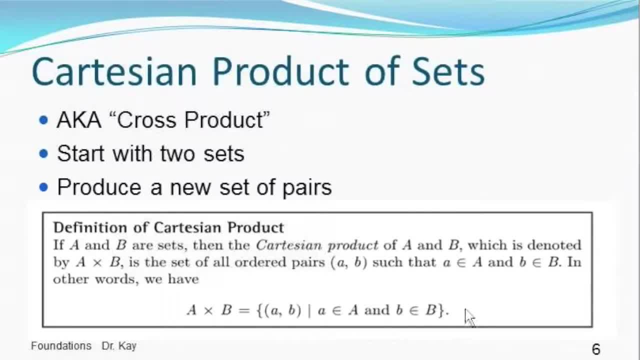 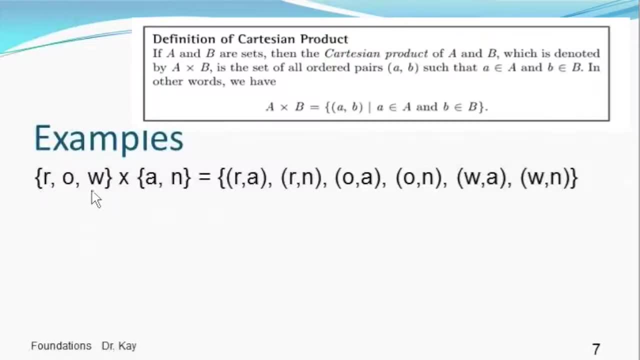 is an element of a and the second element is an element of b. And here's the formal definition of that. For example, if we have two sets, the first set contains three elements- r, o, w, and the second set contains two- a and n- and I take the cross product of those two sets. I end up with this.